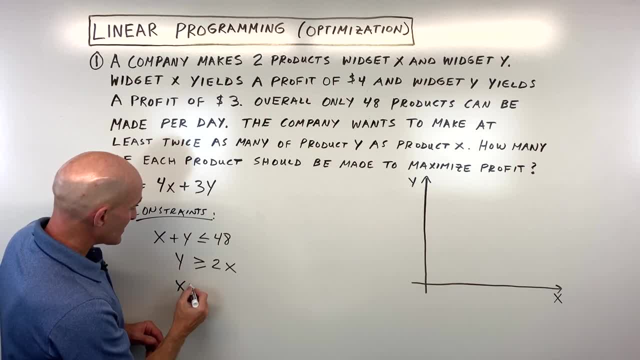 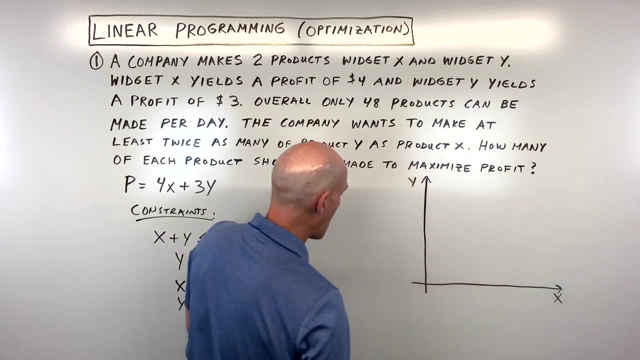 zero. So this is kind of implied that x has to be greater than or equal to zero and y also has to be greater than or equal to zero. Now, x greater than or equal to zero. x equals lines are vertical lines, So greater than or equal to zero would be to the right of the y-axis. 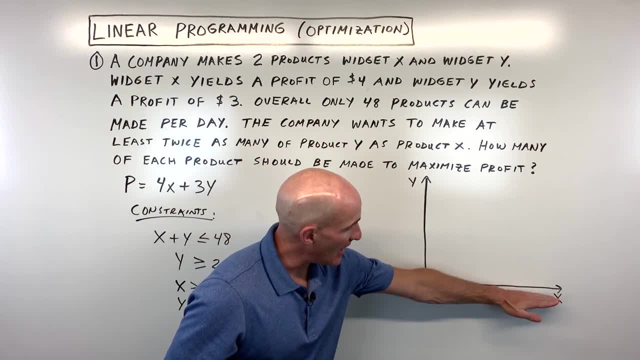 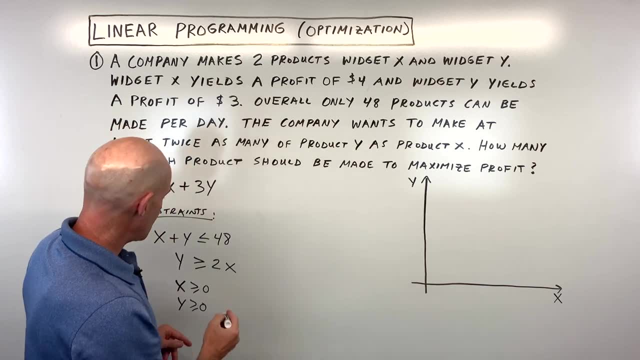 y is greater than or equal to zero. y equals lines are horizontal lines. That's saying greater than or equal to zero is above the x-axis. So that's going to put us here in the first quadrant. So that takes care of these two inequalities. 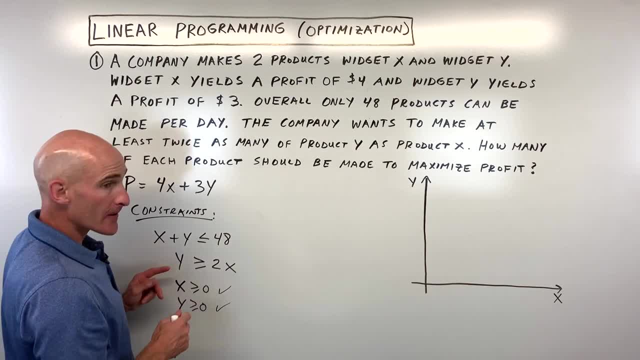 Now let's graph these other two inequalities. So this first one: here you can rearrange this into the y equals mx plus b form, the slope intercept form. Or you can do what we call the intercept method, where you set x to the 0. And that would put y up here at 48.. 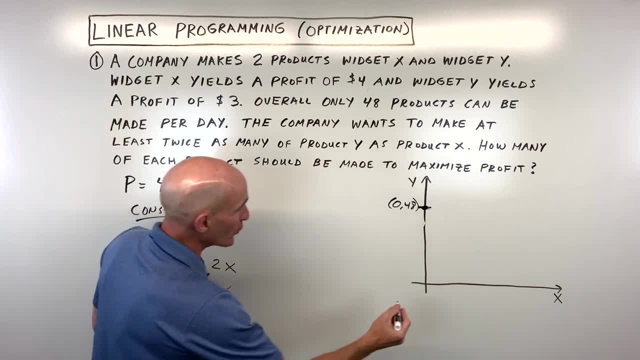 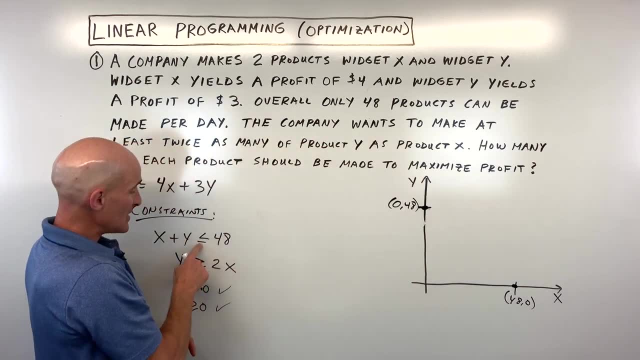 And then if we set y to 0, you can see x equals 48. So let's put that about here. So 48 comma 0. And if we draw a line Now, it's equal to. so that means it's a solid line If it was less than or greater than, but not equal to. 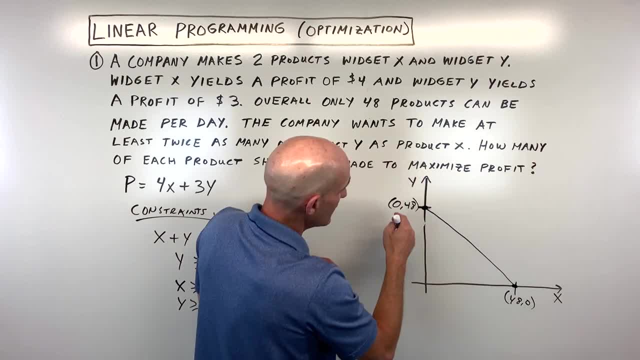 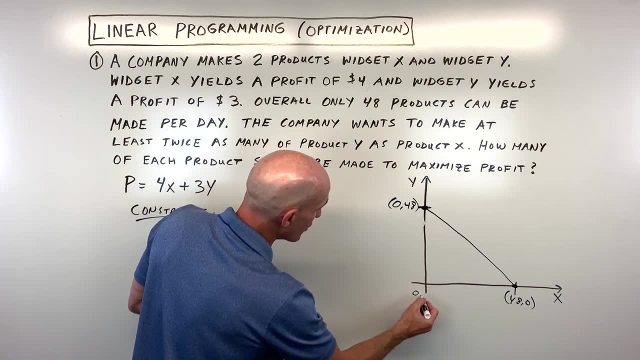 it would be a dashed or dotted line, And I could keep going. but in this case we know we're in the first quadrant point. let's say, for example- I do this origin point here- 0, 0.. 0 plus 0 is 0. Is that less than? 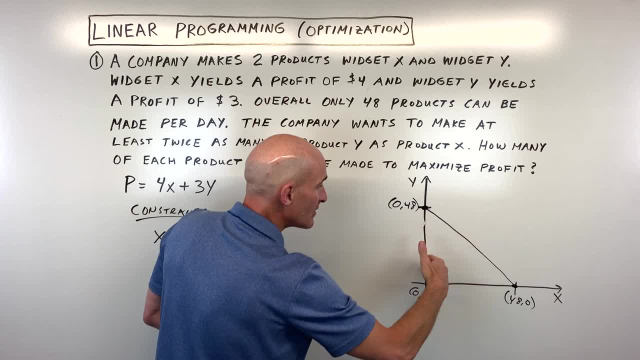 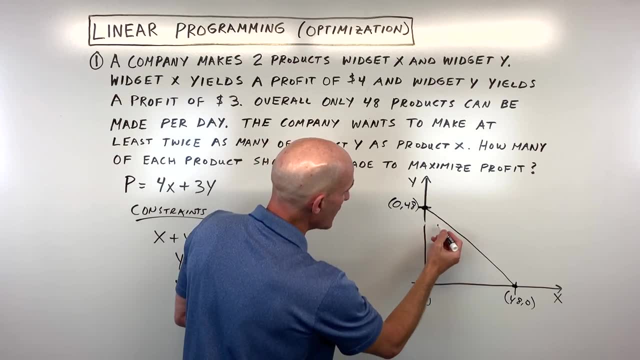 or equal to 48?? Yes, So that means that this side of the line is the true side. This side is the false side. If this was false, we'd shade the other side. So you're just testing to see which side is true. So that's going to put us right here. Okay, so I'll just shade that lightly here. 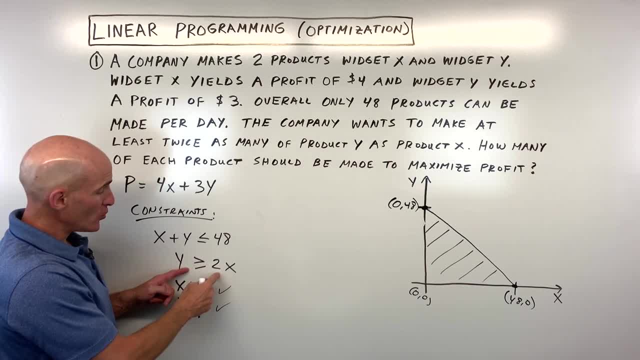 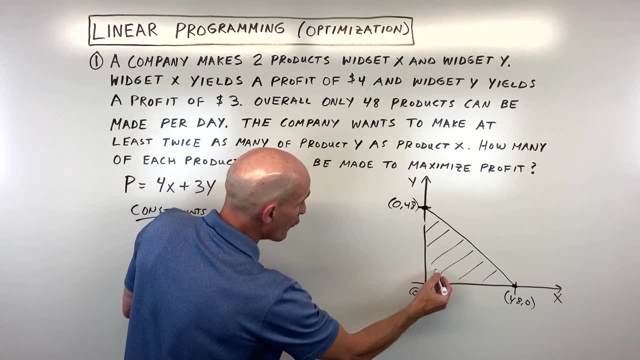 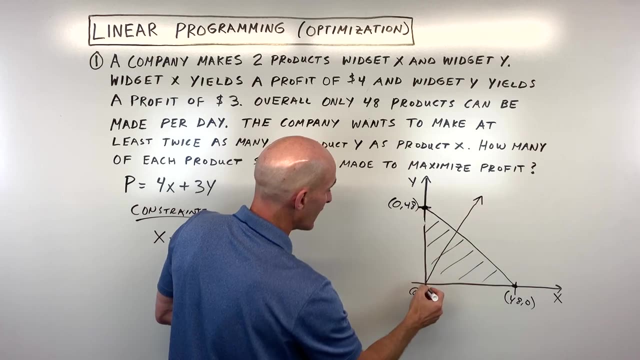 And then for the other inequality, y is greater than or equal to 2x. This is kind of like y equals mx plus b, where b is 0. And we're basically going up 2 over 1, up 2 over 1.. So this is a line that looks something like this, with a slope of 2.. Okay, 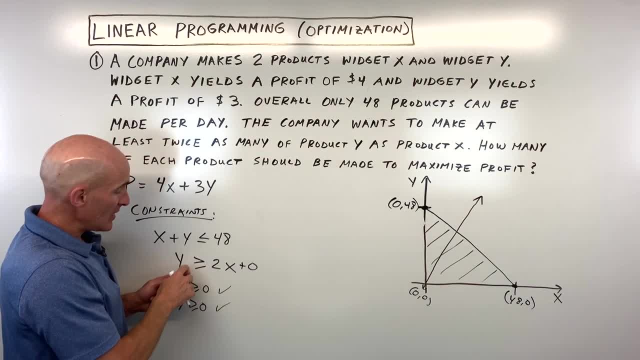 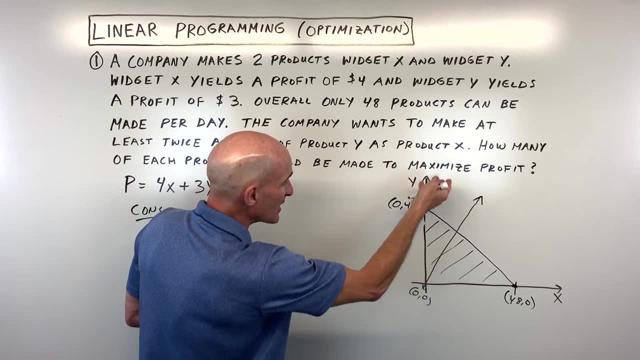 And here, when the y is by itself on one side of the inequality, y controls a vertical direction up and down. So if the y values are greater than or equal to, that means you're going to be shading above this line. So that's going to be on this side of the line, see above. And so that's. 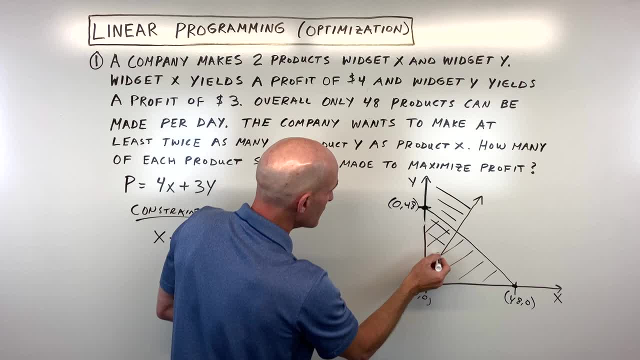 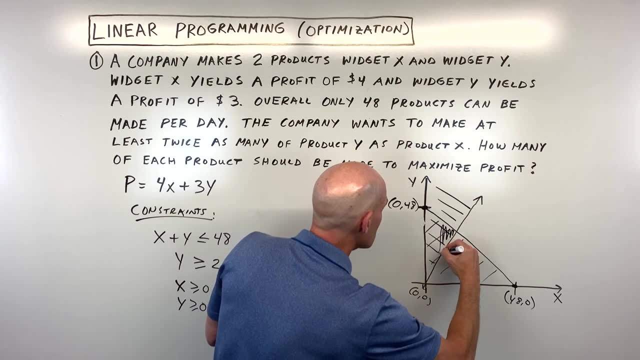 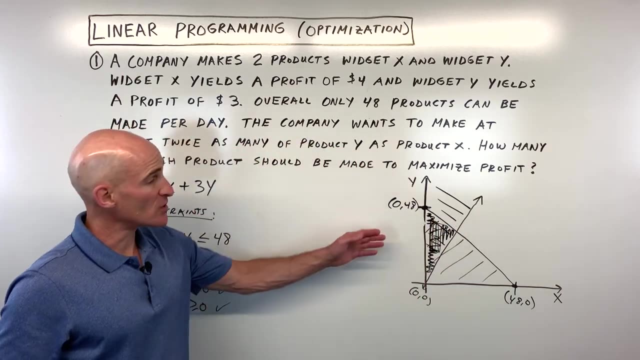 going to put us right there. Now notice that, where are these regions overlapping? They're overlapping right here. I'll kind of shade this in a little bit darker. for us In that triangular region- And this is what's referred to as the feasible region, It's the region that satisfies. 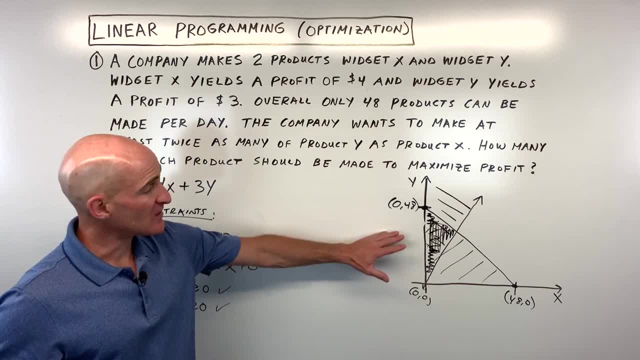 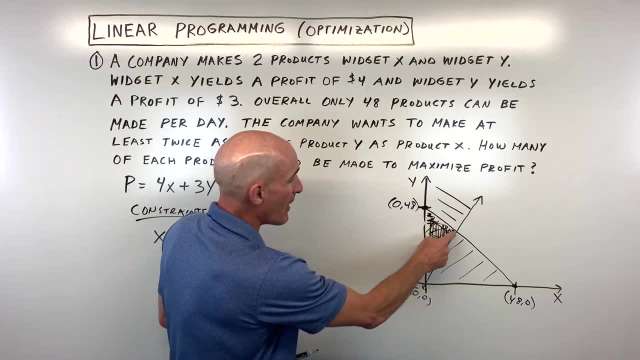 all of our constraints. But what's interesting, once you find this feasible region, your maximum or your minimum is going to be at one of these three points. So you're going to be shading this vertices of this like polygon or the shape that's formed. So what you can do is you can take a look. 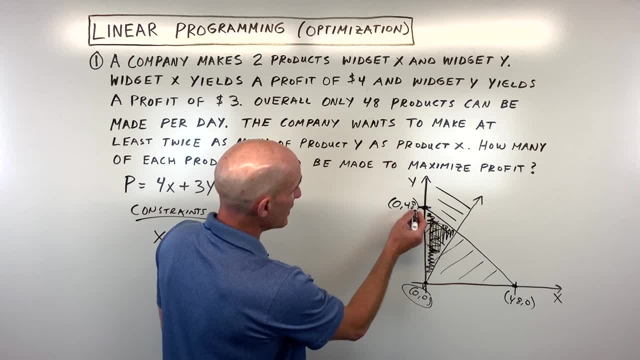 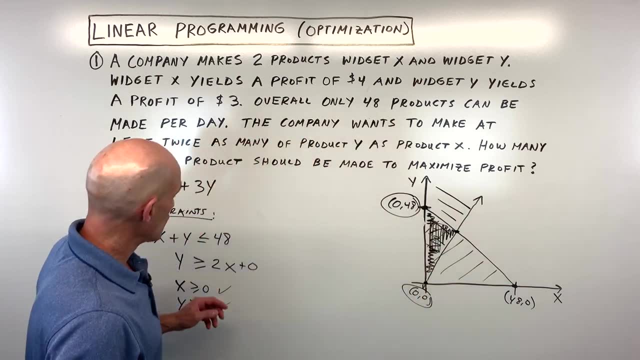 at these points Now. we have this point here is 0, 0.. We have this point here is 0, 48.. But we have to solve for this point right here where these two lines intersect, So we're going to treat these just. 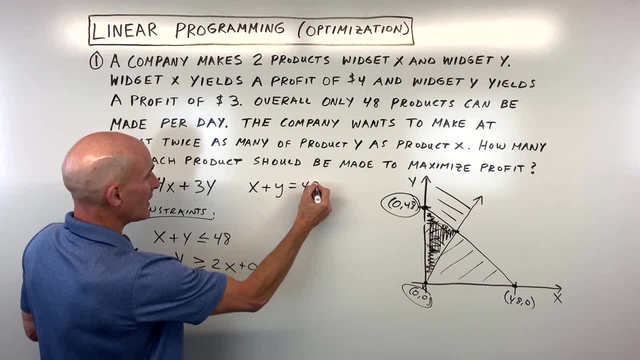 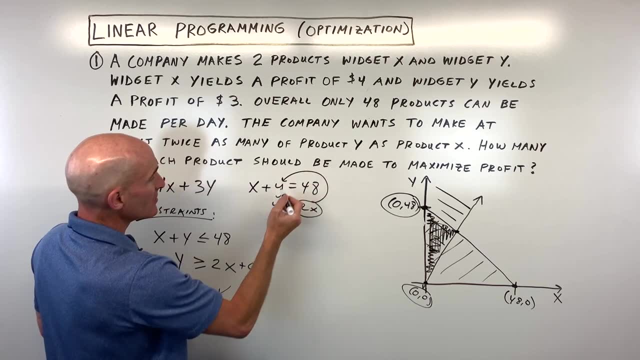 like equations like x plus y equals 48 and y equals 2x, And what we can do is we can do a substitution. So if y equals 2x, let's put 2x in place of y And we can do a substitution. So if 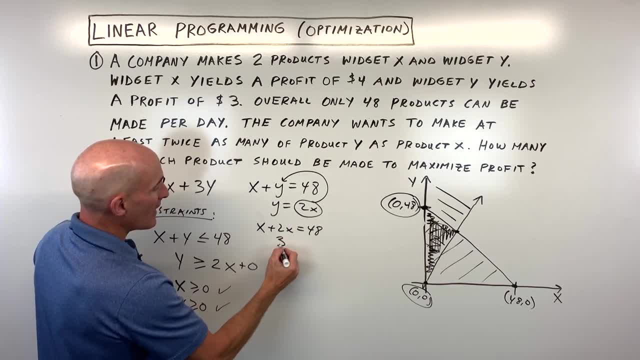 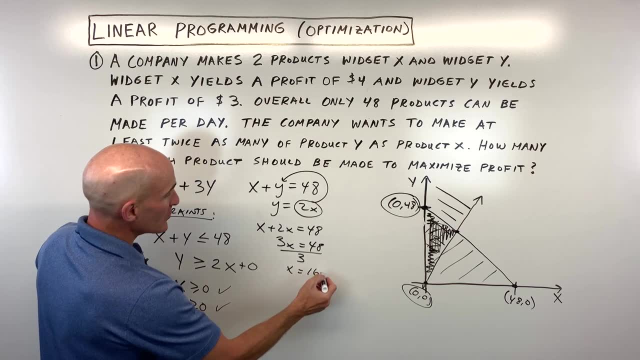 y equals 2x. let's put 2x in place of y, So now we have 3x equals 48. Divide both sides by 3. And you can see that x equals 16.. Now if we put 16 back in here or here, it doesn't matter, You can. 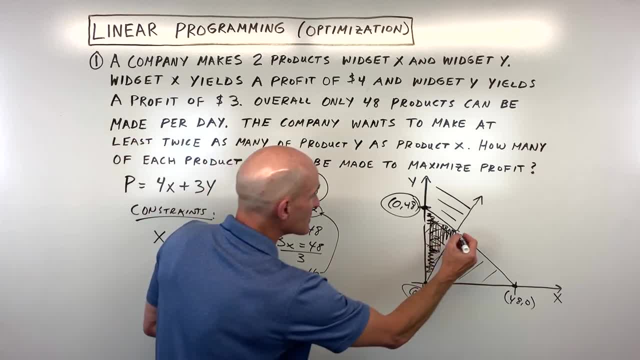 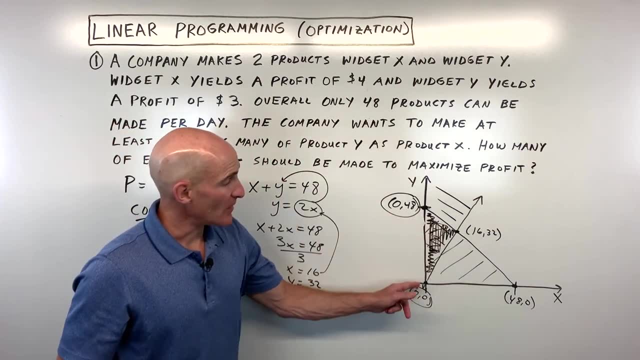 see, y is going to come out to 32.. And so that's the. you know the coordinates of this point. right here is 16 comma 32.. So what we're going to do is we're going to use those vertices of that. 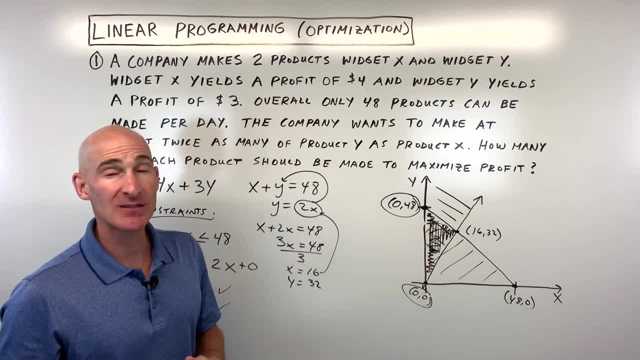 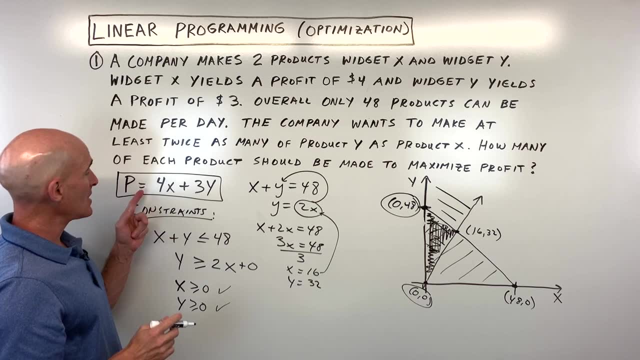 feasible region to see you know which one's going to give us a maximum profit. So let's go back now to our objective function. Okay, our thing that we're trying to maximize or minimize, In this case, our profit, Let's see. Let's take this point here. So if x is 0,, 4 times 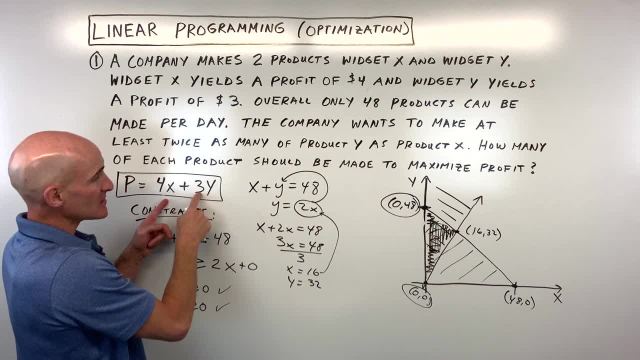 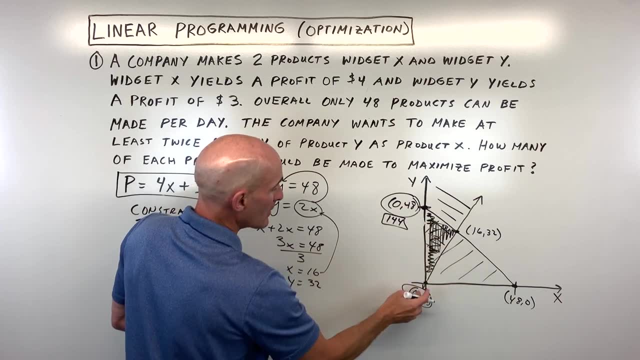 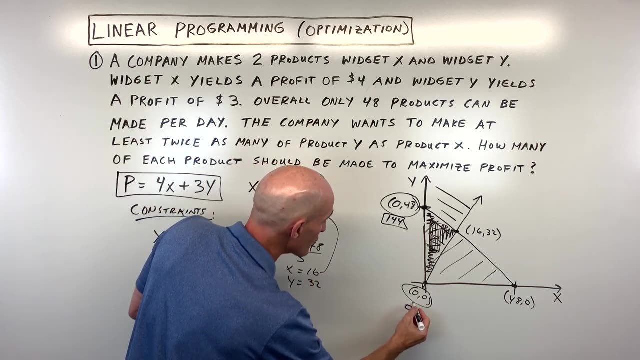 0 is 0.. 3 times 48 is 144.. So 0 plus 144 is 144. for this point, Let's do 0, 0 next. 4 times 0 is 0.. 3 times 0 is 0.. 0 plus 0 is 0.. So this one's going to be 0 here, which makes sense If you. 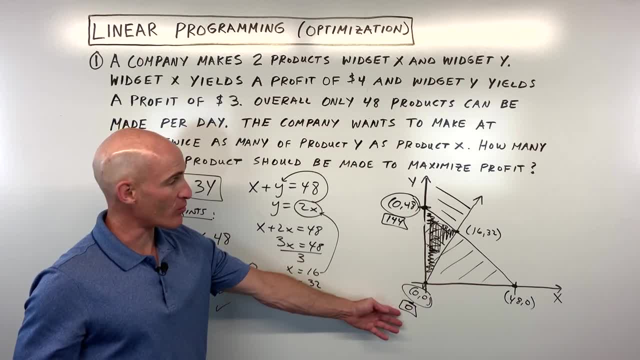 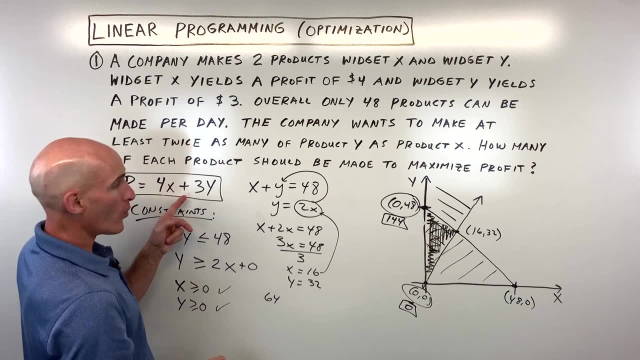 sell, or if you make none of the either of the products, you're going to have a 0 profit. And let's check this point here: 16, 32.. 4 times 16 is 64. And 3 times 32 is 96. And if we add that, 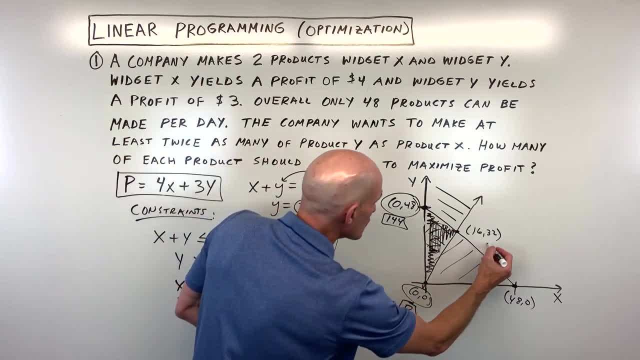 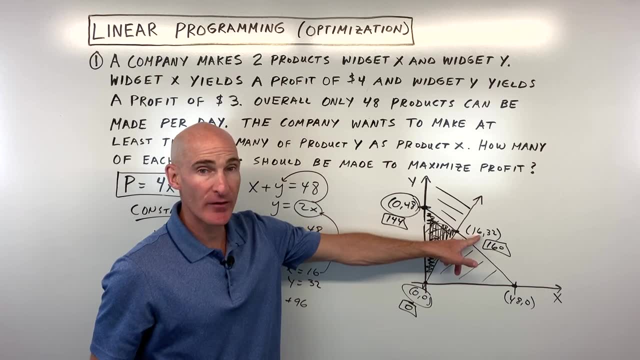 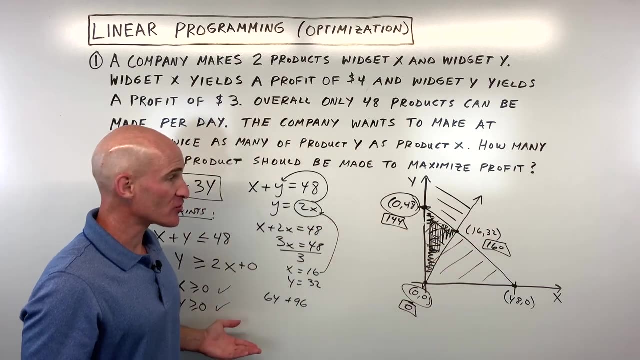 together, let's see that's 160.. So what that tells us is that this is giving us the maximum profit of $160 if we manufacture 16 of product x and 32 of product y. So we're going to have a of product y and that'll satisfy our constraints but yet maximize our profit. So let's take a look. 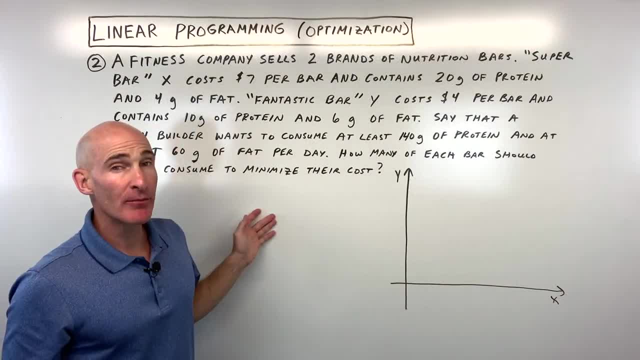 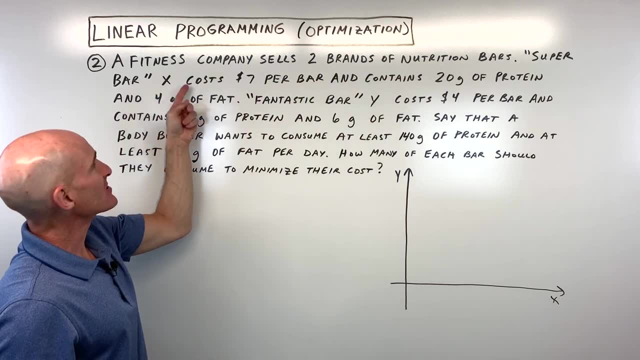 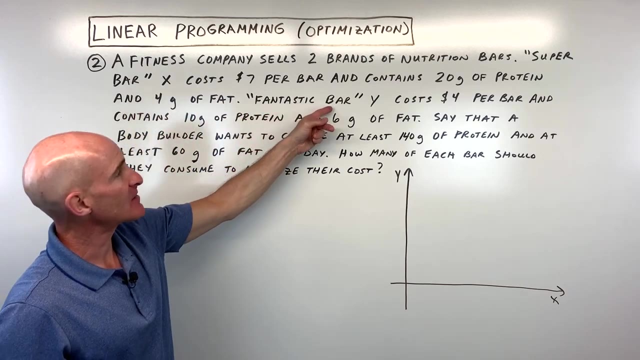 at another example where we're trying to minimize something. Okay, for example number two, let's dive into this one. It says a fitness company sells two brands of nutrition bars. Super Bar X costs $7 per bar and it contains 20 grams of protein and 4 grams of fat. Fantastic Bar Y: 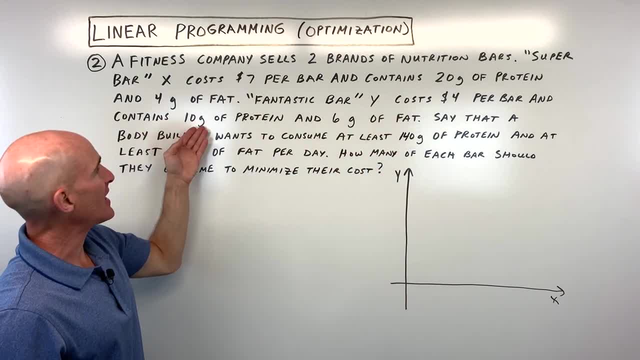 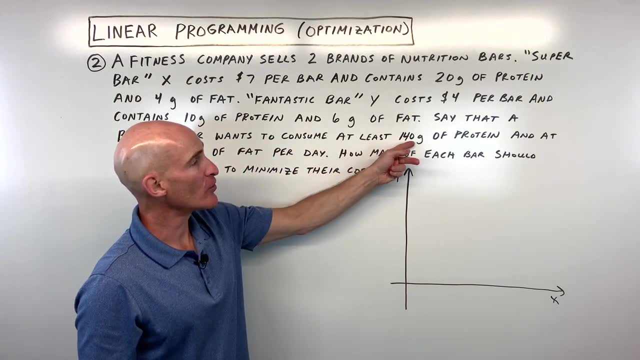 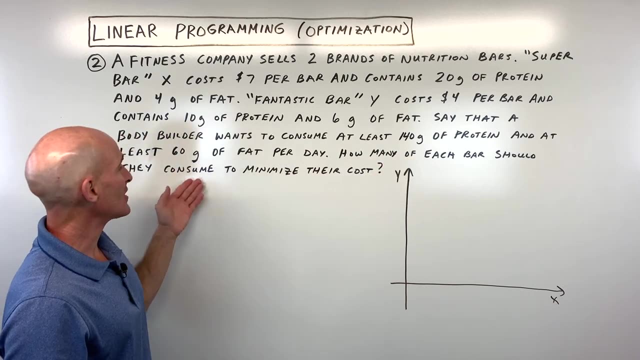 costs $4 per bar and it contains 10 grams of protein and 6 grams of fat. Say that a bodybuilder wants to consume at least 140 grams of protein and at least 60 grams of fat per day. How many of each bar should they consume to minimize their 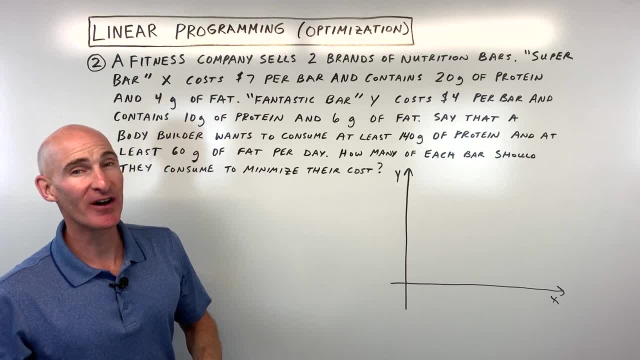 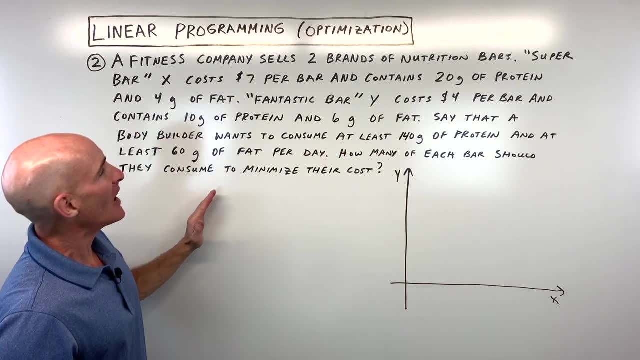 cost Okay. so before we do this problem- this isn't nutrition advice- Make sure you talk to your doctor or a nutritionist to find out what you should actually eat here. But in this particular problem, let's go ahead and figure out what we're trying to minimize. We're trying to minimize. 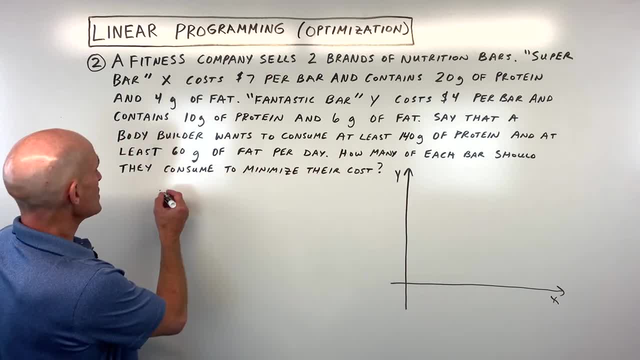 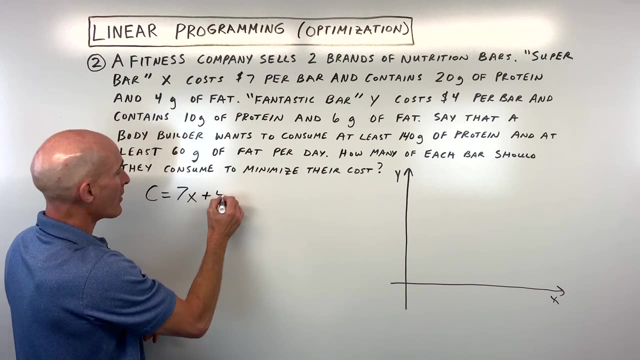 the cost. So let's write that objective function first. So the cost is what? It's $7 for Super Bar X, So $7 times the number of the Super Bar X, plus it's $4 for Fantastic Bar Y. So this is going to: 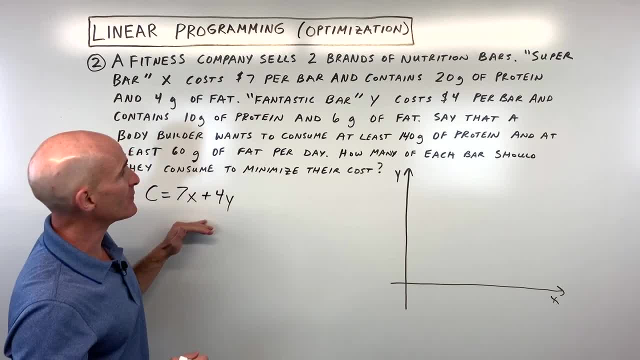 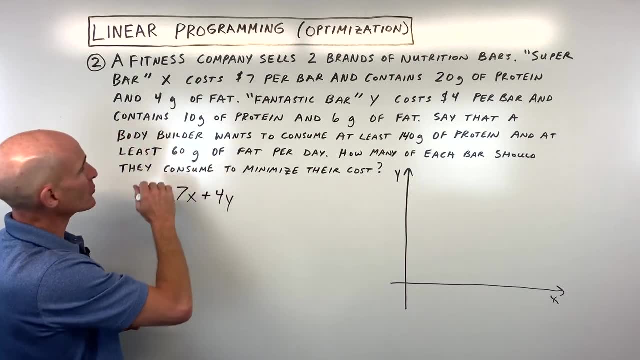 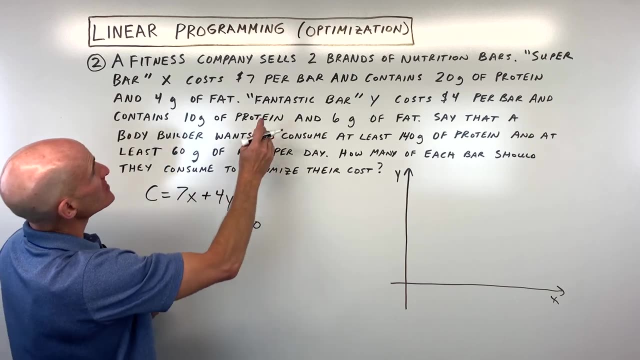 be the cost equation. This is what we're trying to minimize. okay, our objective function. Now let's look at our constraints like kind of the restrictions here, And the restrictions are that the bodybuilder person wants to consume at least 140 grams of protein per day, But it looks like 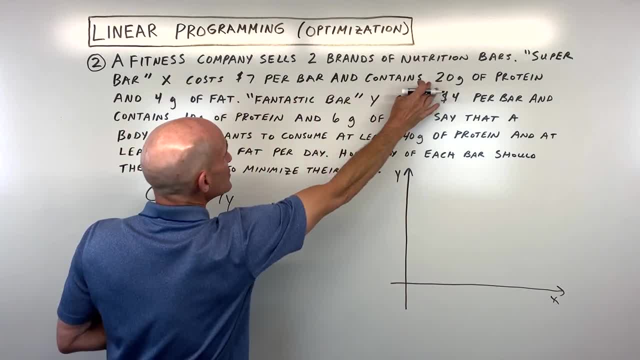 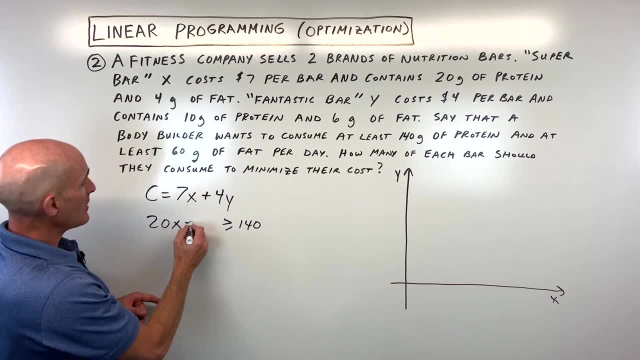 the first bar, Bar X, contains 20 grams of protein, So that's 20 grams times the number of that X brand nutrition bar. plus the Fantastic Bar Y, it contains 10 grams of protein. So that's going to be 10 times Y, Okay, and when you add that up it's going to be 10 times Y. So that's. 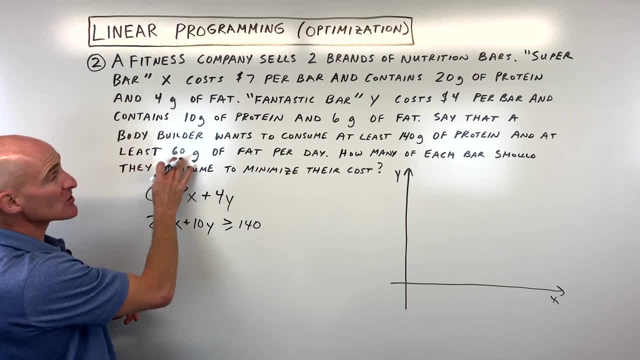 going to be 10 times Y, So we're going to have to get that together. that has to be greater than or equal to 114.. Now the fat. they also want to consume at least 60 grams of fat per day, So at 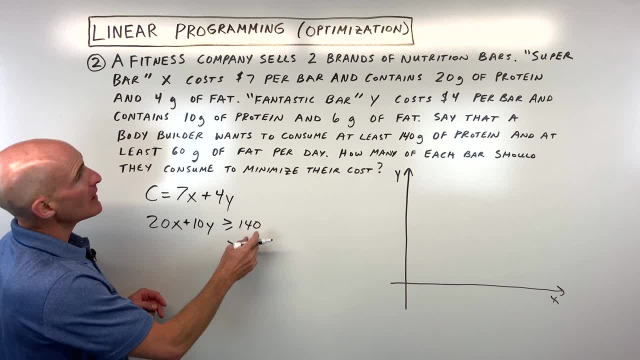 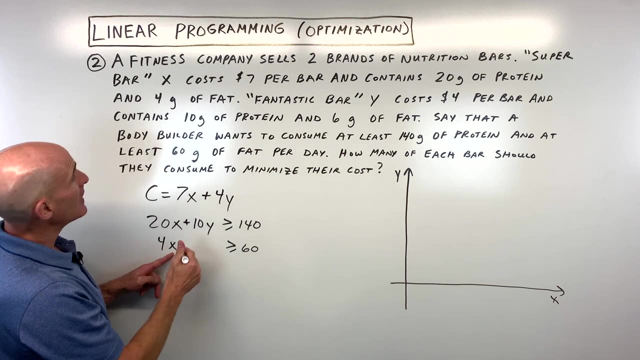 least means greater than or equal to 60 grams. And it says that the first bar, Bar X, Super Bar X- it contains four grams of fat, So four times the number of bars here you're going to get. let's say you consume five of these, that'd be 20 grams of fat. And for Fantastic Bar Y, that contains 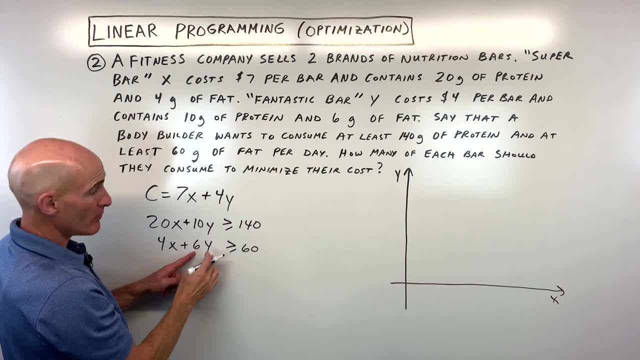 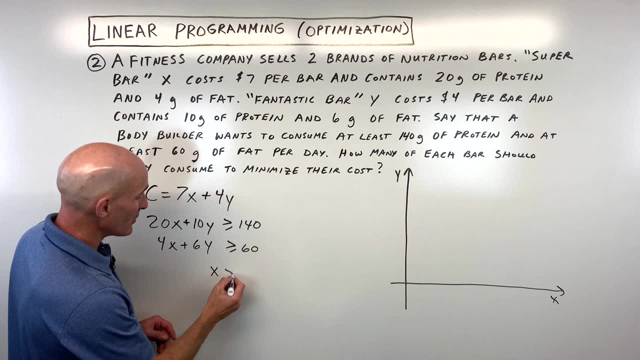 contains six grams of fat. So six times the number of bars here you're going to get, let's say you number of bar Y. Okay good, so now we also have to take into account those implied domains that you can't really consume: a negative number of each bar. so 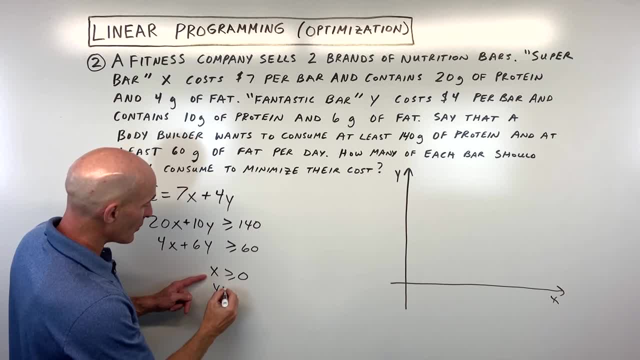 it has to be greater than or equal to 0 for bar X and greater than or equal to 0 for bar Y, which again that puts us into the first quadrant here. Okay, so we took care of those two constraints. Now let's plot these Now generally, when the 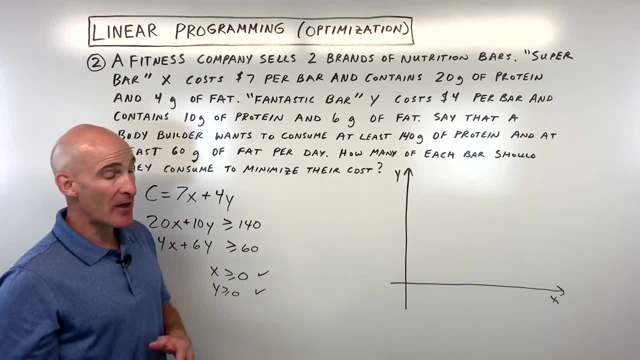 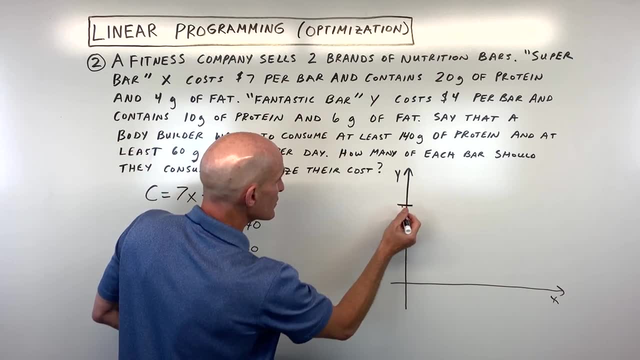 variables are on the left side of the inequality. I like to do the intercept method, where I set X to zero and solve for Y. So if X is zero, here you can see Y would be 14.. So let's just say this is 0 comma 14.. If Y is 0, 0 times 10 is 0.. 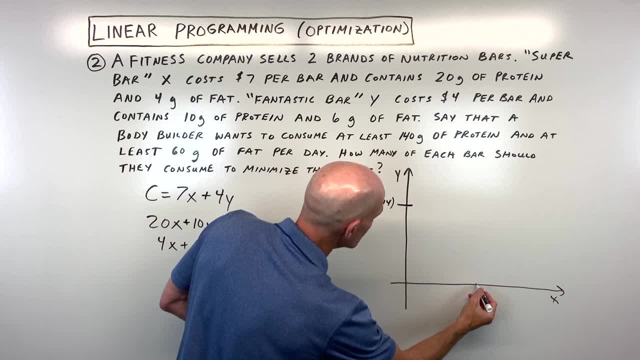 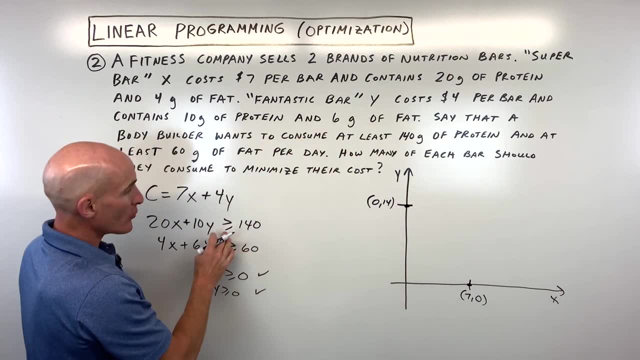 Divide both sides by 20, you can see that X is coming out to 7.. So let's just say this is 7: 0 here, And this is a greater than or equal to. So equal to means it's a solid line And I can do it, the test point method. So 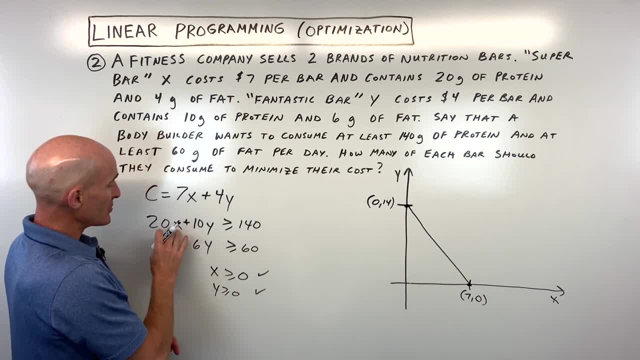 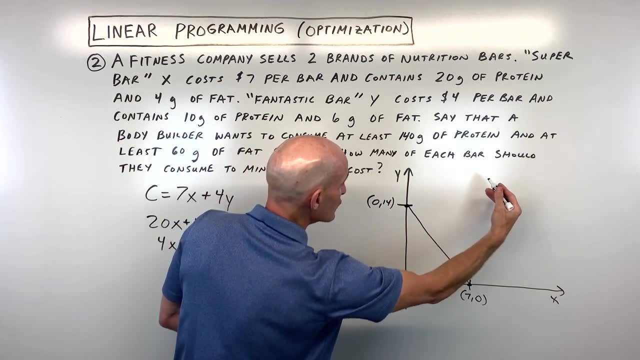 if I put 0 in there, there will be zero, and then if I put 7 in there, there will be zero. our origin in here that's going to be zero plus zero is zero. is that greater than or equal to 140? no, so this is the false side of our line. the true side would be this side, so we can shade. 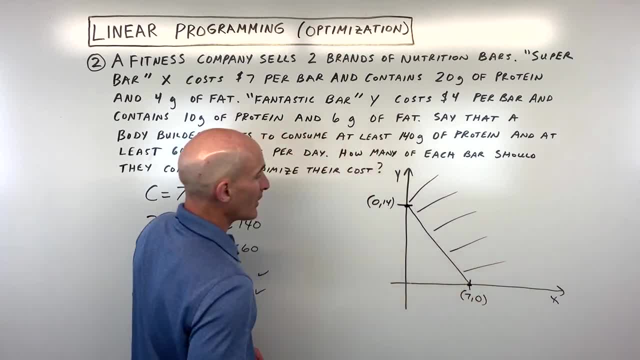 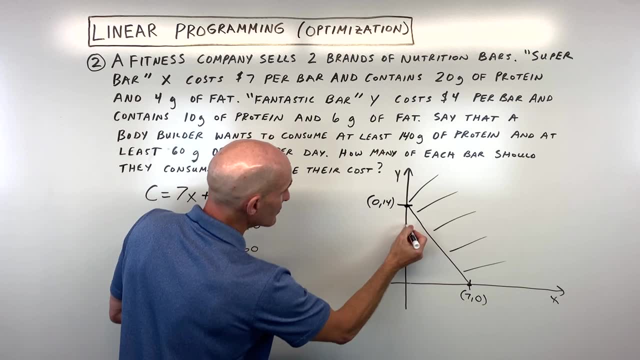 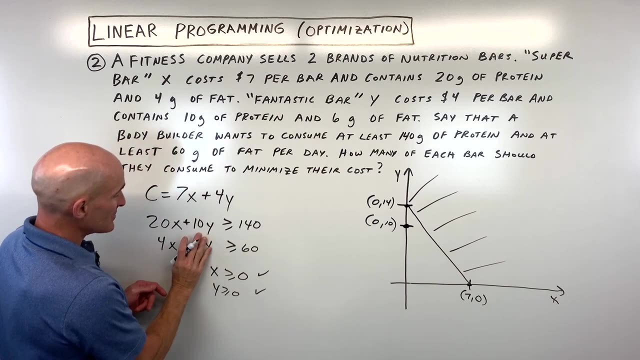 like that. okay. and then the other inequality. let's do the same thing. if we set x to zero, divide by six, you can see y is 10, which is going to be somewhere over here. and if y is zero, six times zero is zero. divide both sides by four, you can see x is 15. 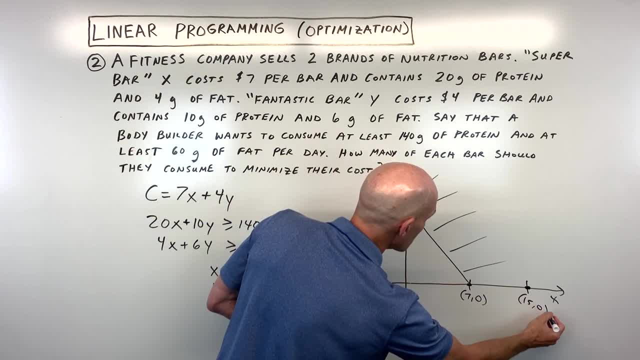 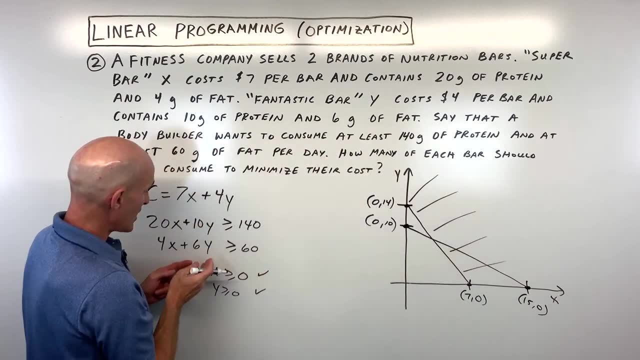 some way, somewhere, way over here and again, we have greater than or equal to. so equal to- it's a solid line- greater than. let's double check. now. what we want to do is we want to do a test point. so we pick zero, zero. that's going to be zero plus zero is zero. is that greater than or equal to 60? 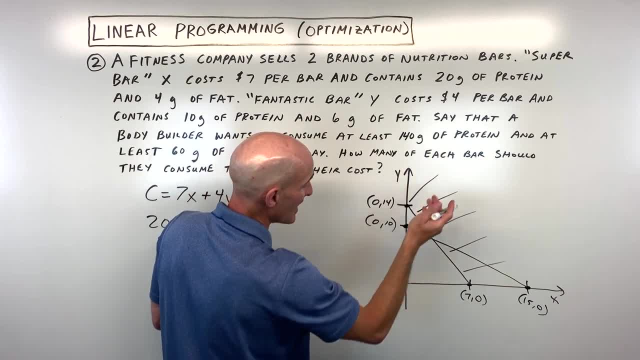 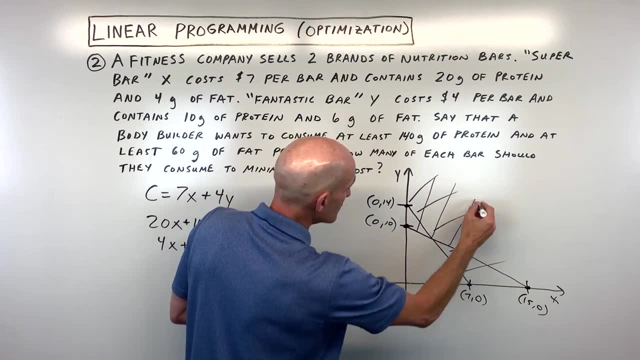 no, so this is the false side. we want to do a test point, so we pick zero, zero. that's going to be zero. we're going to shade on the other side of this line, so that's going to be right here. okay, and so now what we're looking at is: where do all these 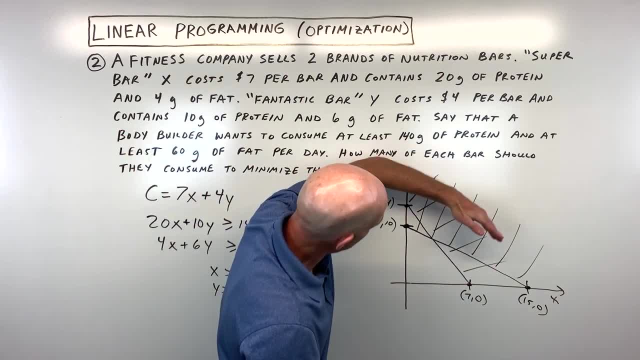 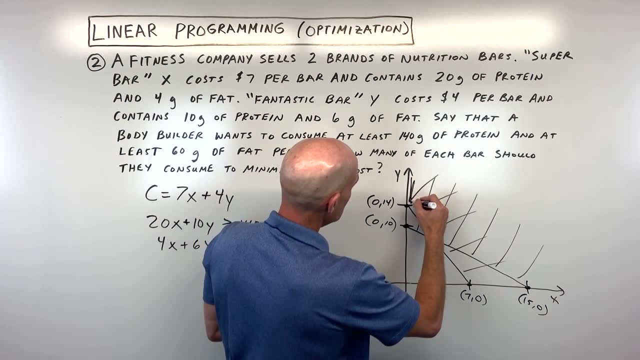 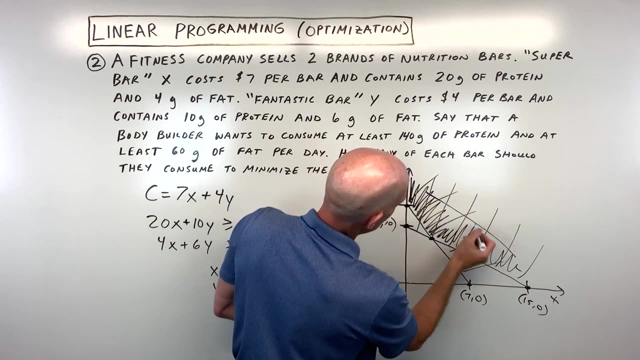 inequalities overlap. well, you can see, we're above this line. we're above this line. so our shaded region here, our what's called our feasible region, is going to be right here. so i can shade that in here a little bit darker for us. so basically it's like kind of this shape here. 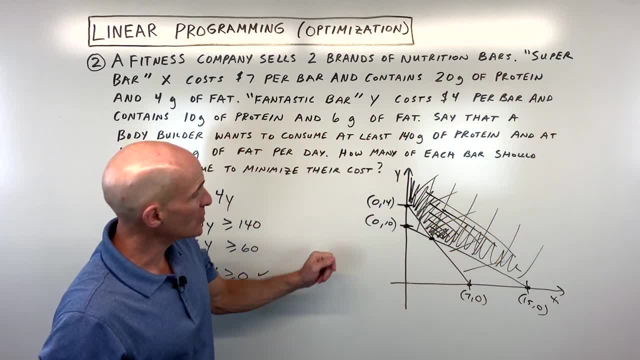 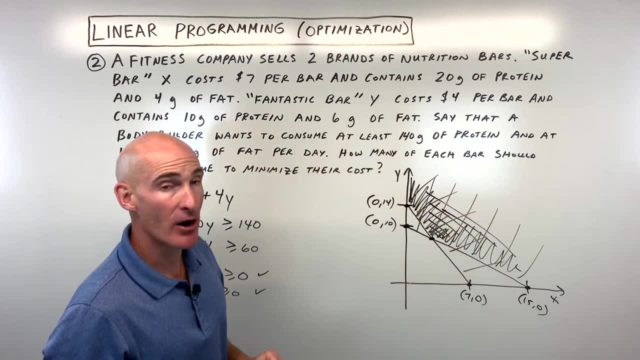 and going out, right, but we're trying to minimize the cost. so what we're going to do is we're going to test this point, this point right here and this point right here that's going to satisfy our constraints, but then we can see which one's going to minimize our cost. let's find out what. 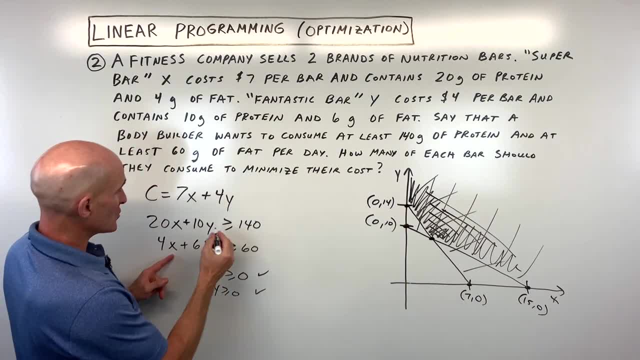 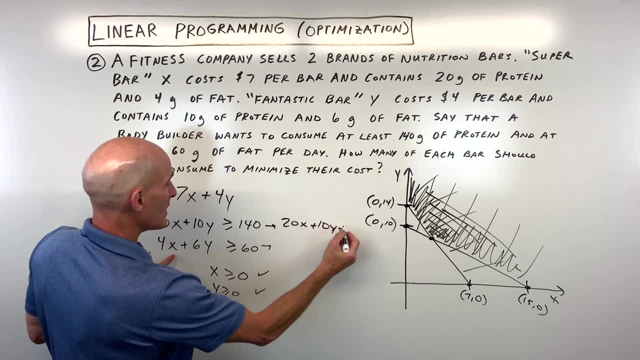 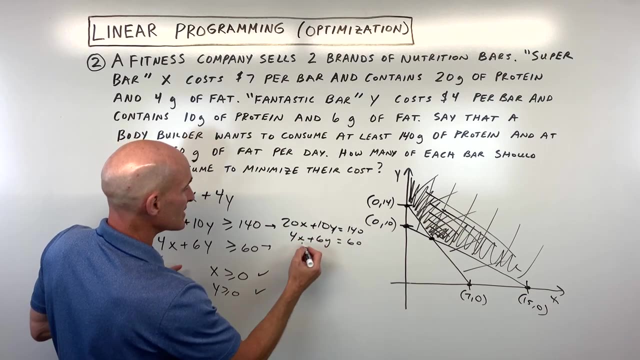 this point of intersection is here. we're going to have to solve a system of equations, so we're going to treat these just like they're equal signs. we're going to say 20x plus 10y is equal to 140 and this equation here, 4x plus 6y, is equal to 60. now what we can do is we can. 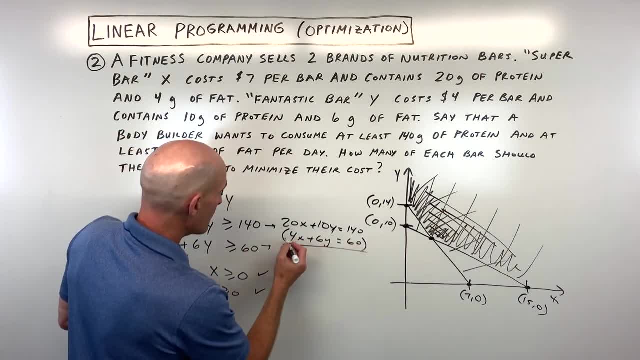 multiply this bottom equation by negative 5, and the reason i'm doing that is because that'll give us a negative 20x, and when i add it to this top equation, the x's will cancel each other out. so this would be minus 30y equals negative 300. so let's add these equations together: the x's cancel. 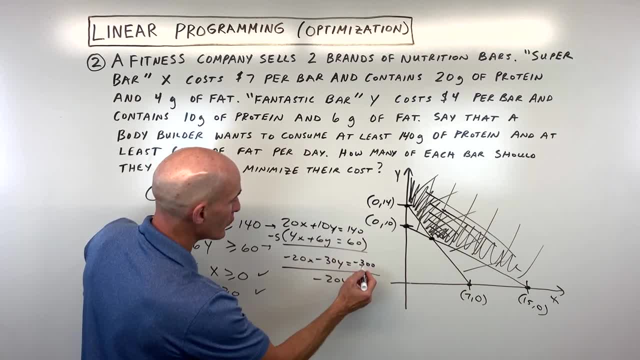 10y plus negative 30y is negative 20y. 140 plus negative 300 is negative 160, and if we divide by negative 20, y is coming out to 8. now if we take the 8, we can put it back into either equation. 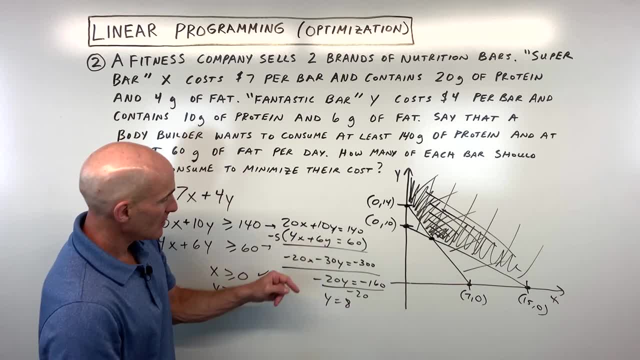 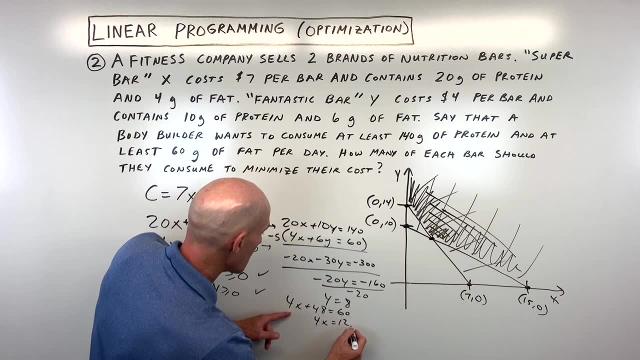 i'll do this one here: 6 times 8 is 48. okay, so that's 4x plus 48 is equal to 60. subtract 48 from both sides, 40 4x equals 12. divide both sides by 4 and x is coming out to. 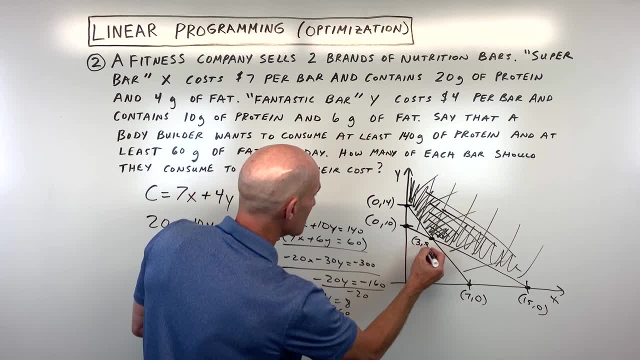 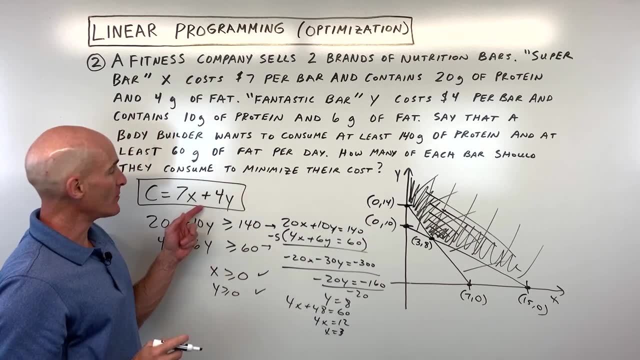 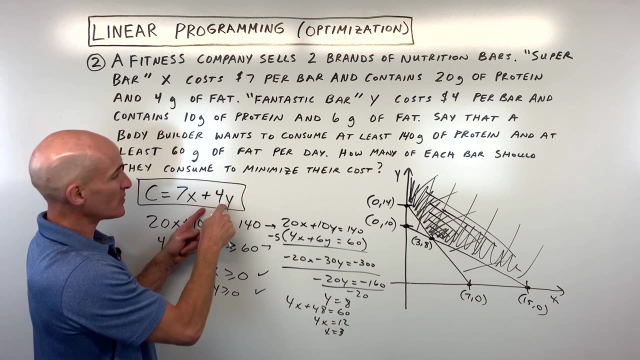 3, so this point right here is the point 3, comma 8. so let's go ahead and test those points now into our objective function. we're trying to maximize or minimize, and let's start with this point here. so 7 times 0 is 0, 4 times 14 is 56, 0 plus 56 is 56. so what that means is it would cost. 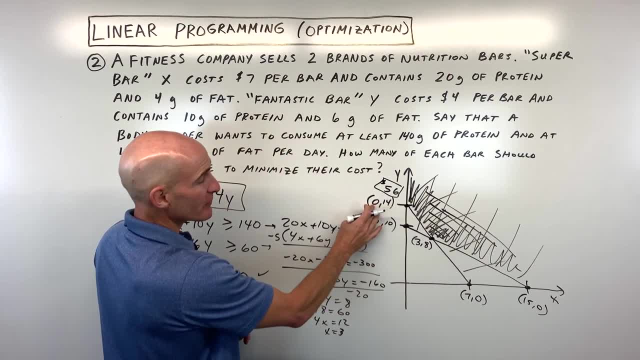 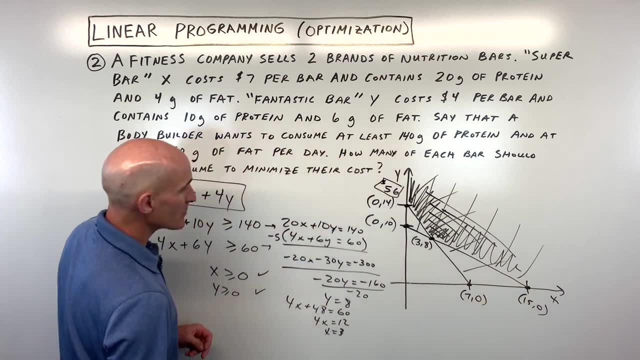 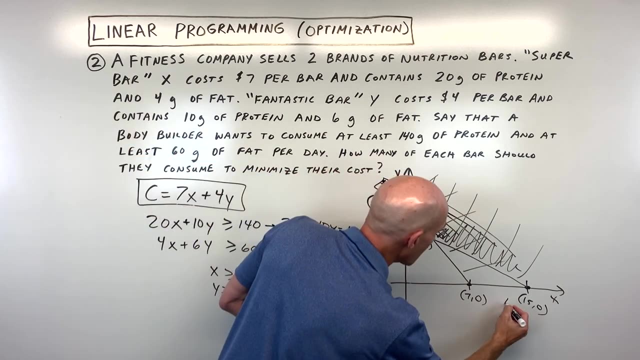 56 dollars to consume 0 of nutrition bar x and 14 of nutrition bar y. let's go down to this point here: 15, 0, 7 times 15 is 105, 4 times 0 is 0, 105 plus 0 is 105. so it costs. 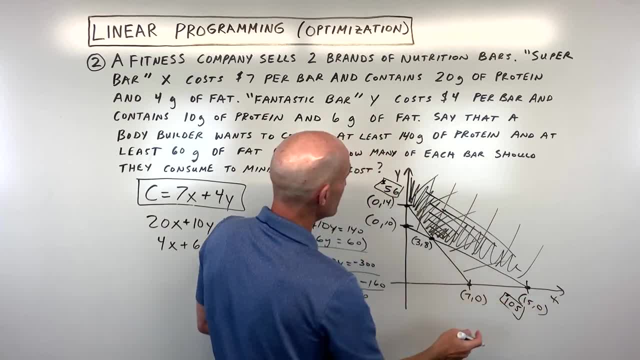 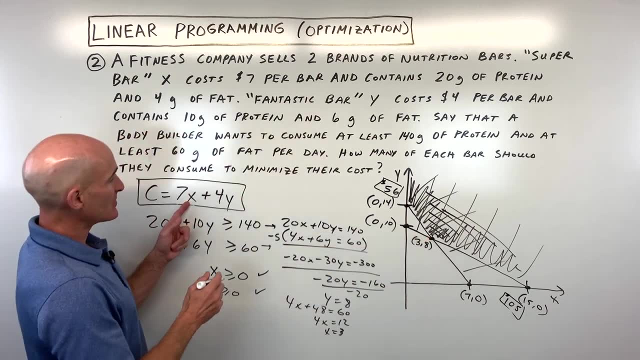 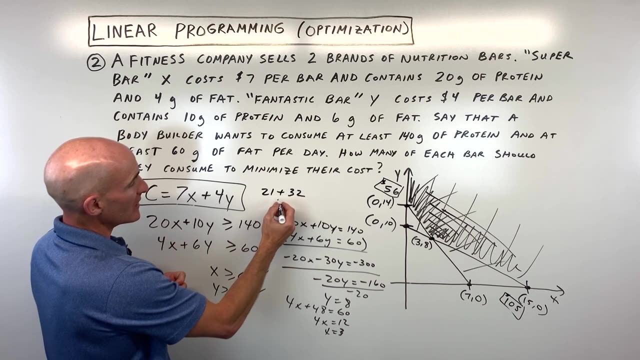 105 dollars if you consume 15 of nutrition bar x and 0 of nutrition bar y, and then here at this point, 3, 8, 7 times 3 is 21, 4 times 8 is 32. if we add those together we get 53. so this: 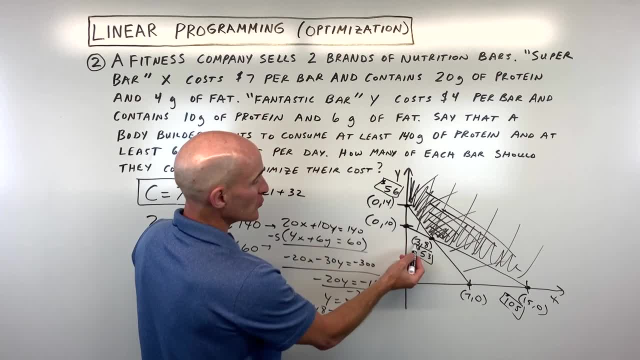 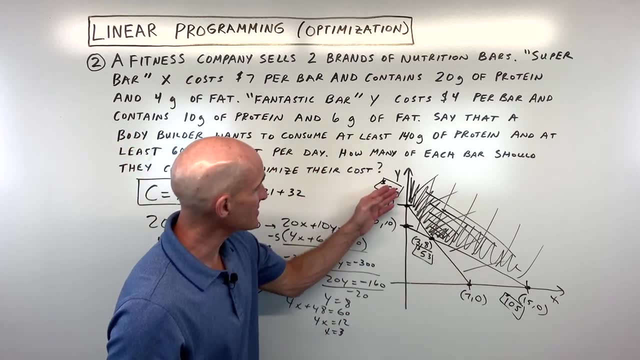 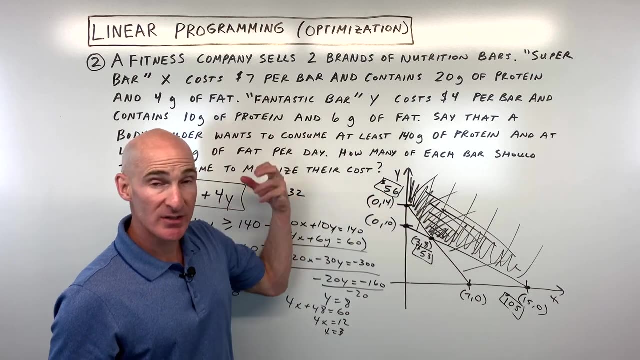 one is costing 53 dollars. if we consume 3 of nutrition bar x and 8 of nutrition bar y, which one's giving us the lowest cost? it looks like this point right here: 53 dollars would be 3 of bar x and 8 of bar y, to satisfy all the constraints but yet minimize the cost now. 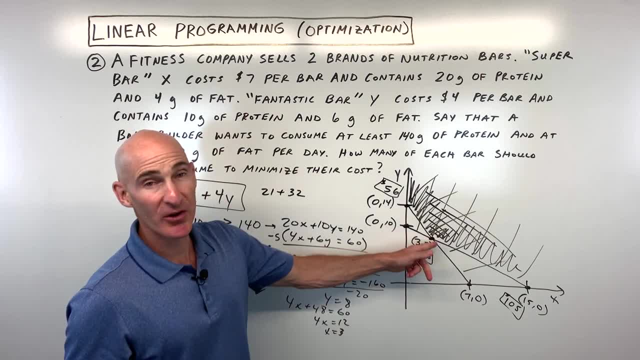 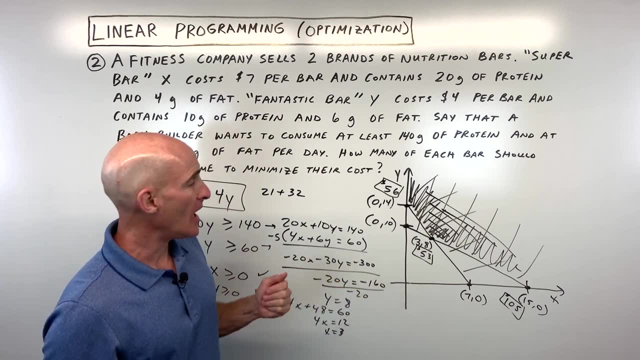 you might be saying, mario, isn't it always the one in the middle? well, it really depends on the problem, it depends on the objective function, it depends on your constraints. it really depends, uh, but you want to check each of the points that are on the vertices of that.